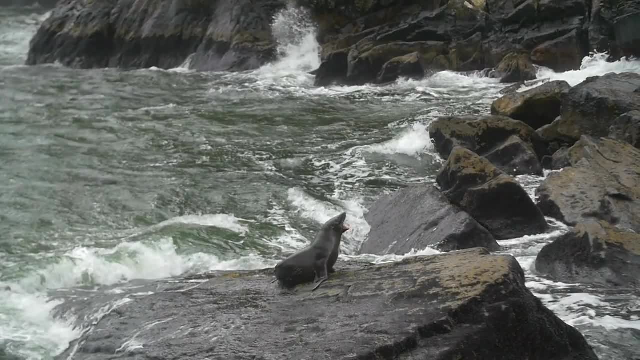 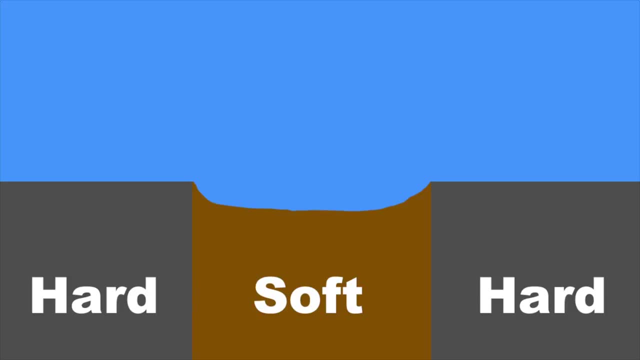 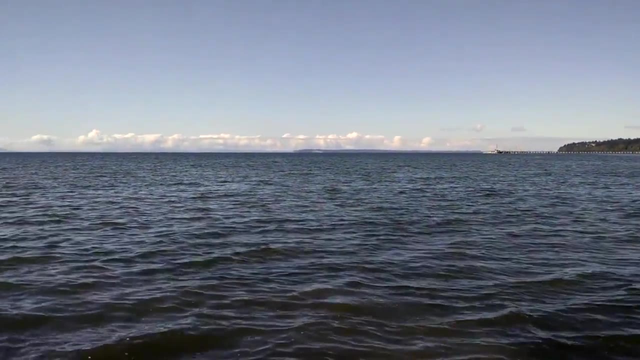 A bay forms when rock is eroded, But not just any rock rock that is relatively soft Compared to the rock beside it. the softer rock erodes at a faster rate, which recedes the coastline. As you can see, White Rock Beach is on a bay. 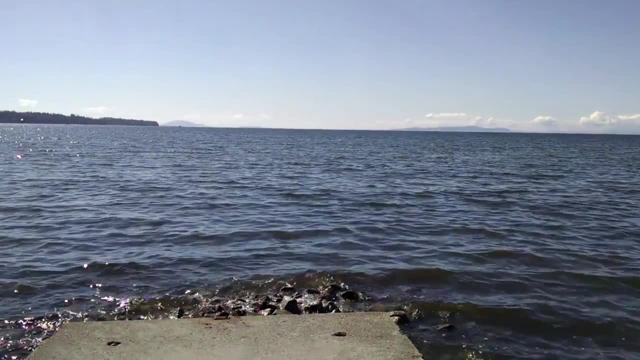 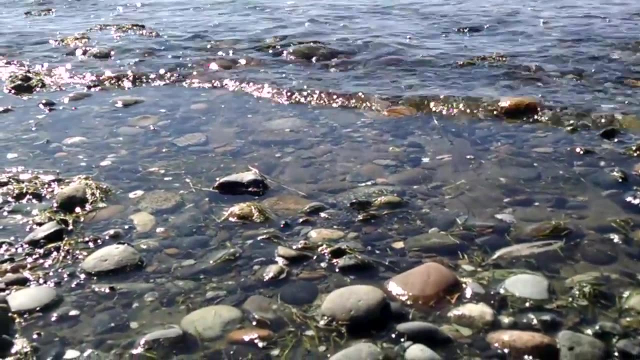 The pieces of land sticking out are called headlands, which are made of harder rock than the bay. Another criteria for a beach is that the swash, which is the incoming wave of water, is stronger than the backwash, the retreating water. 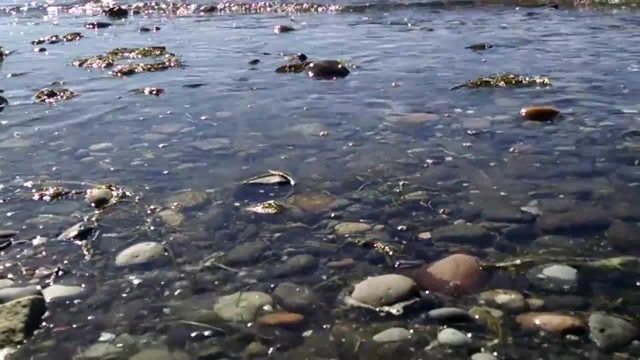 The swash is an area of the beach that is relatively soft. The swash is an area of the beach that is relatively soft. The swash is an area of the beach that is relatively soft. The backwash is extremely evident, while the backwash isn't quite as obvious. 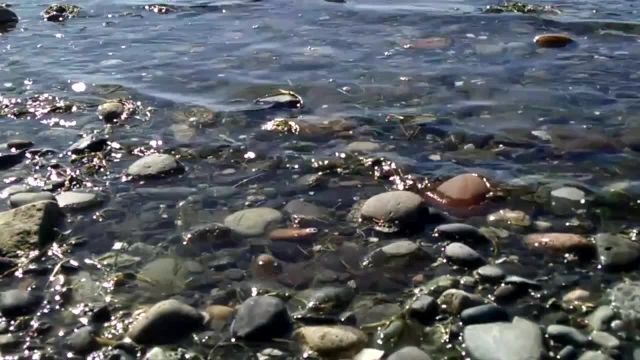 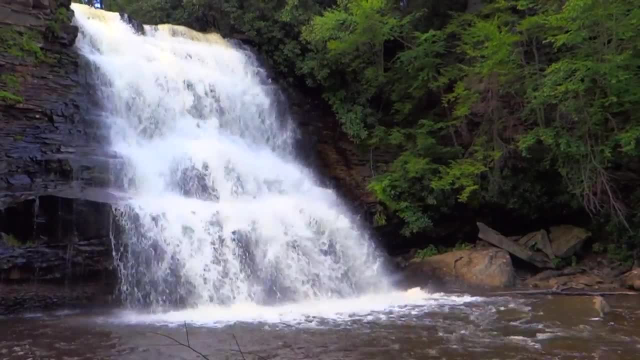 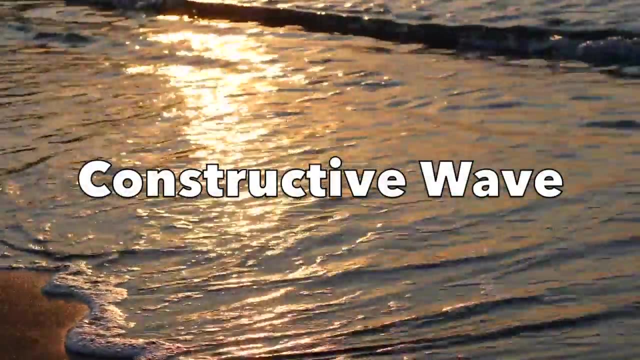 On a diagram it seems simple enough, but the forces of nature, especially when viewed in real time, are rarely simple. Water is a good carrier of loose material, which is exactly what beaches are made of. If the swash is stronger, the wave is called a constructive wave. 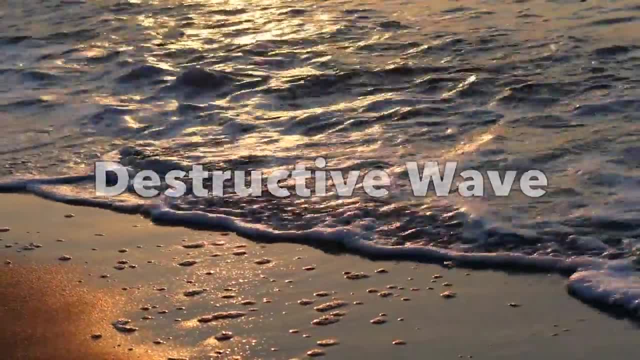 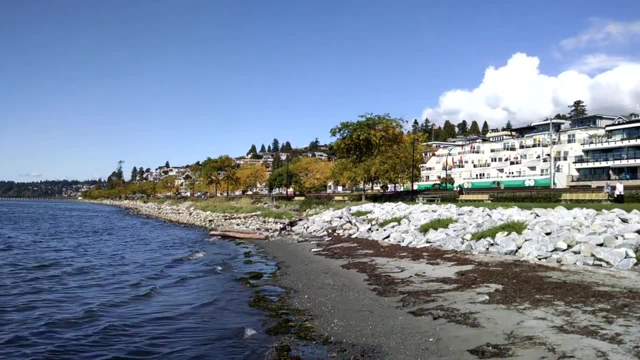 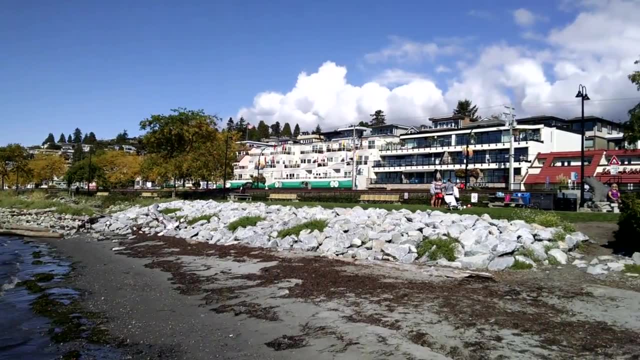 The waves are constructive. The waves are constructive. All you have to do to confirm this is proof by contradiction, when we assume the opposite is true, and look for contradictions. If we assume the wave is destructive, then there would be no natural beach. 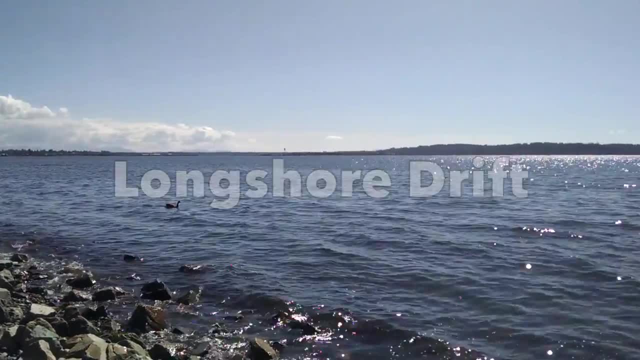 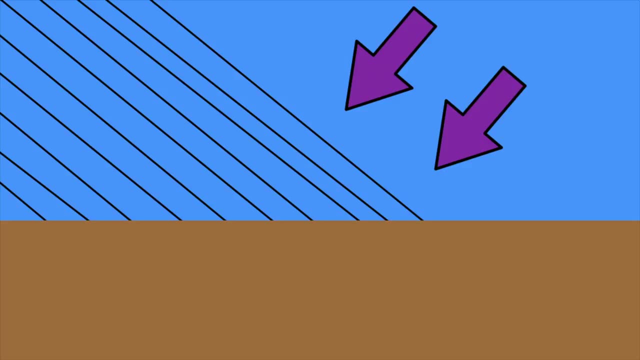 The wind, water and sediment result in another phenomenon called longshore drift. As you may have noticed, the wind rarely blows perpendicular to the shore. Thus the swash comes in at an angle. But regardless of the angle of the swash, the backwash always moves at a 90 degree angle. 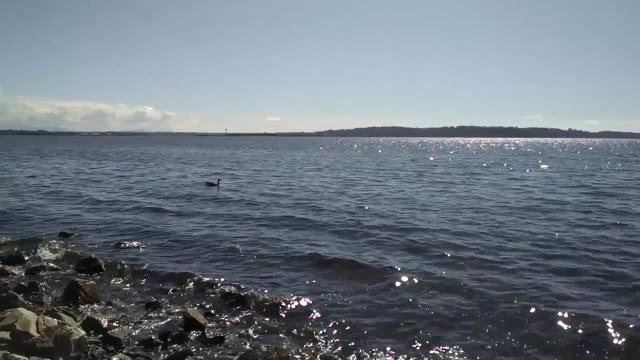 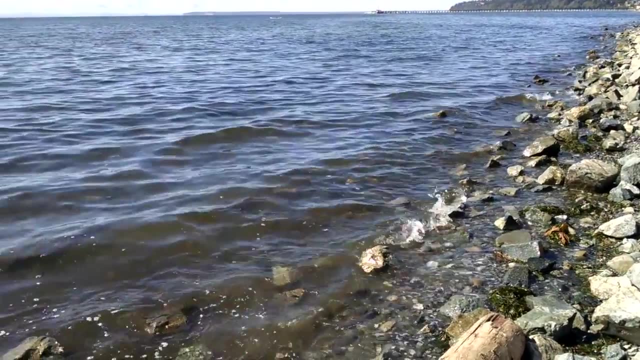 90 degree angle to the shore. If this process is repeated over and over, sediment moves along the shore. This isn't necessarily obvious, unless it's what you're looking for. So if the wind is blowing south more than north, as it is here in White Rock, the loose 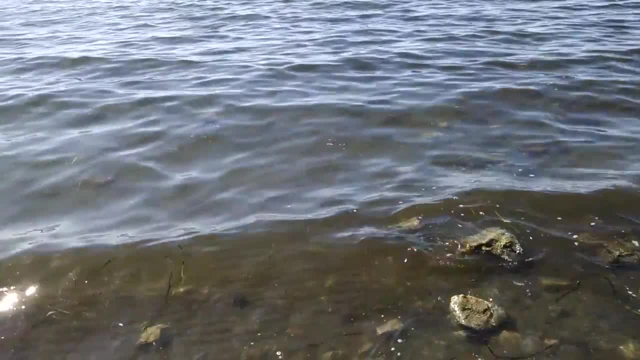 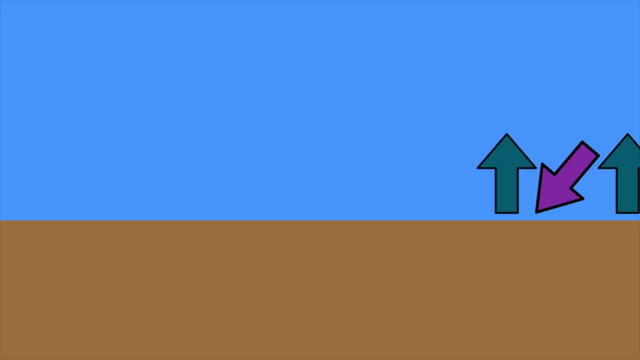 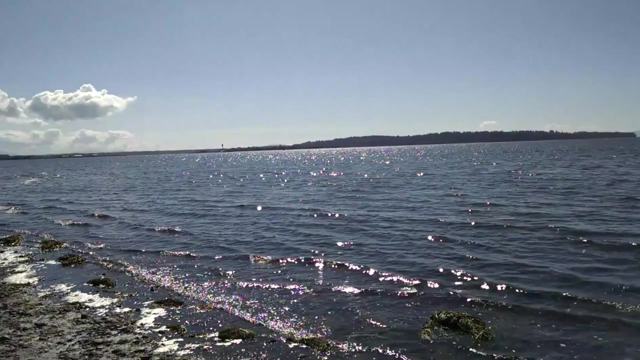 material moves south. An interesting feature which arises from longshore drift is a spit. Basically, a spit forms when longshore drift carries sediment and compiles it into a piece of land which sticks out into the ocean. You see that water tower over there. 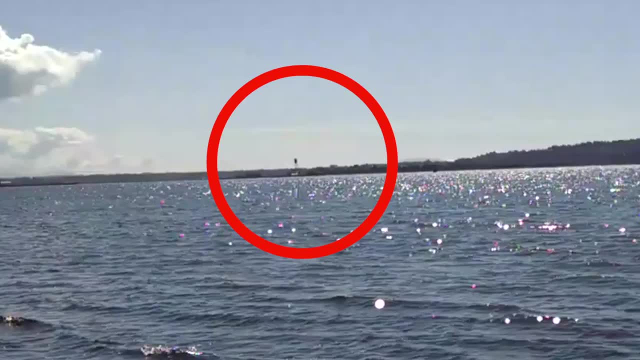 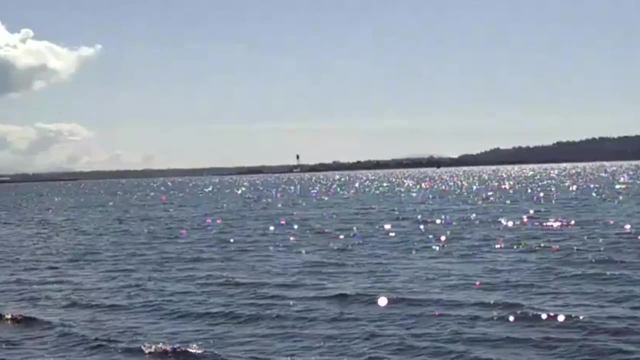 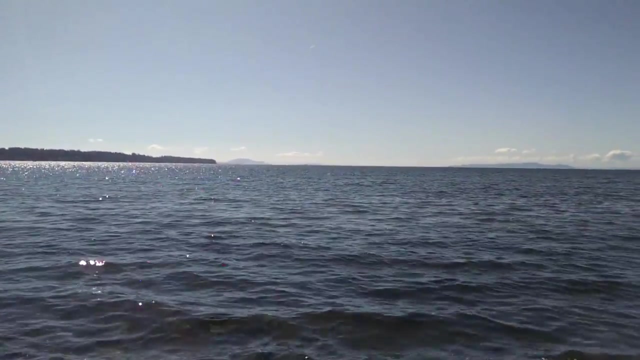 That was built on a spit In another country. Since it's a result of longshore drift, spit formation relies on the wind direction, which influences ocean currents along with swash and backwash. It's interesting how I could travel for kilometers in my country minding my own business and 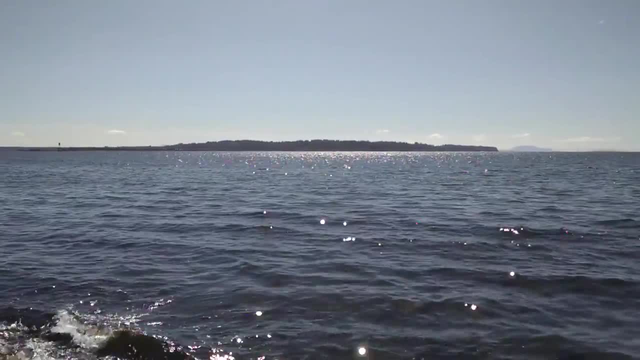 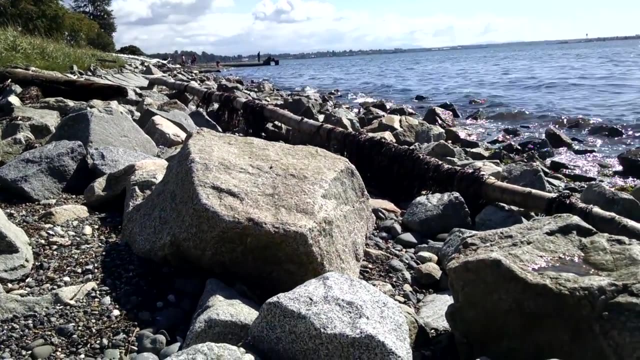 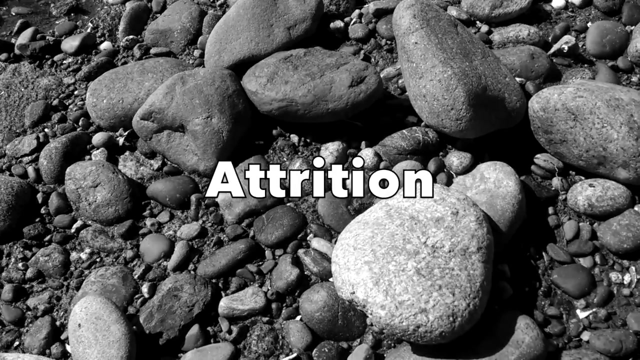 nobody has to care. But if I cross this little body of water Again, I'm doing my own business. Then suddenly a lot of people start caring. But how do things erode? How do rock and other solids wear away? Well, firstly there's attrition, which is when rocks strike each other. 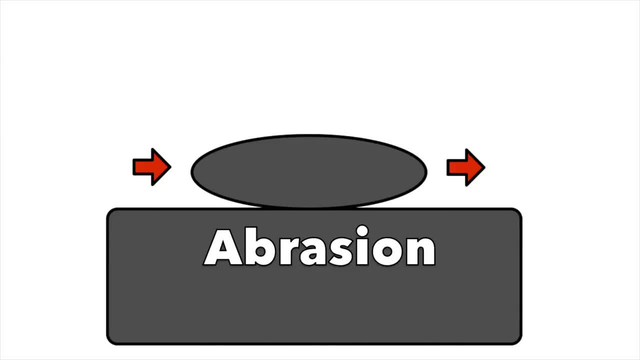 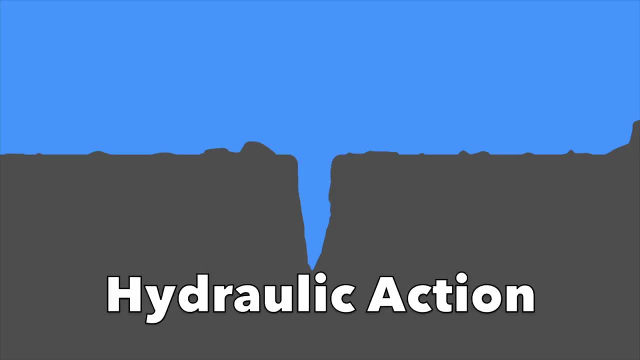 Abrasion is when they rub together. This can also happen with sediment, which is easy enough to spot here, as the water is full of sand. Hydraulic action, in which water is driven into cracks. Finally, there's corrosion, Which is a chemical breakdown. 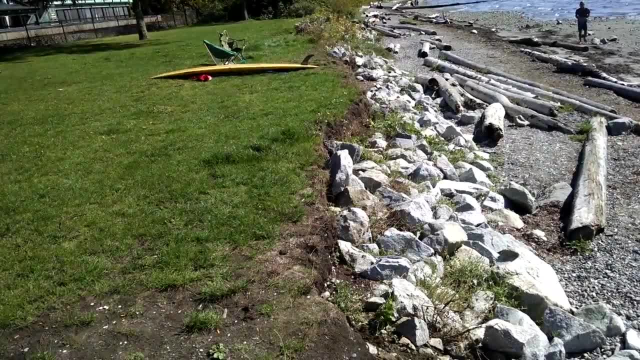 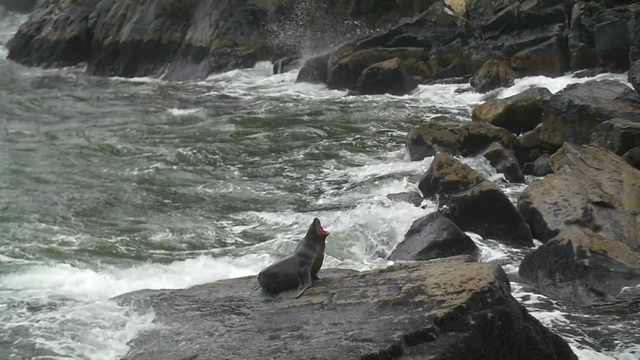 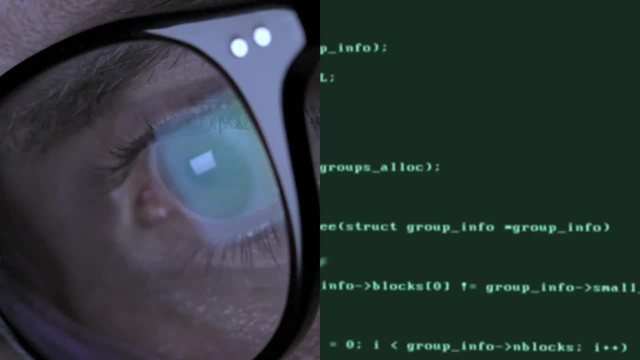 Usually erosion isn't noticeable overnight, but it can happen. Do we sit back and let nature have the last laugh? Well, yes, We have no system that defends against nature entirely, But we're humans, so with our intelligence we find ways to slow down natural processes. 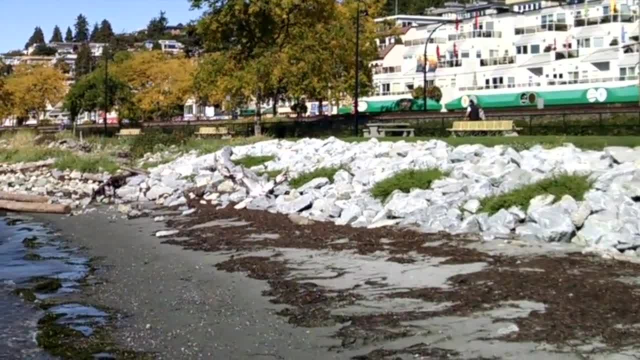 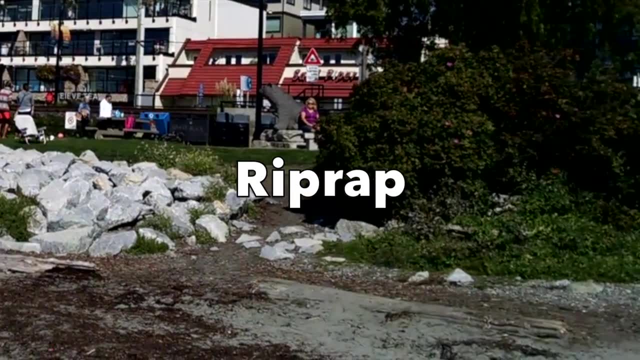 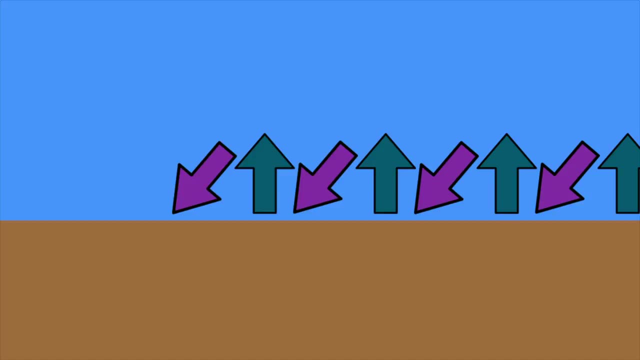 To protect against erosion, rocks are placed above the high tide limit. If you ever go to a beach and see rocks like these, they're not natural, They're called a riprap. Now back to our good friend, longshore drift. To protect against longshore drift stripping beaches away, groins are installed. 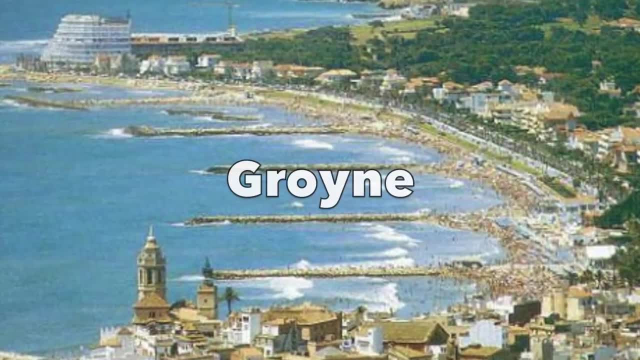 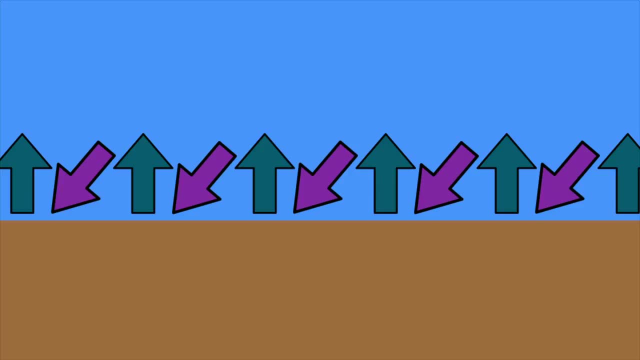 Not this type of groin but that type of groin. Since longshore drift causes sediment to move along a coast in the same direction as the wind, beaches can lose sand. To prevent this, groins are installed to trap the sediment from moving along the beach. 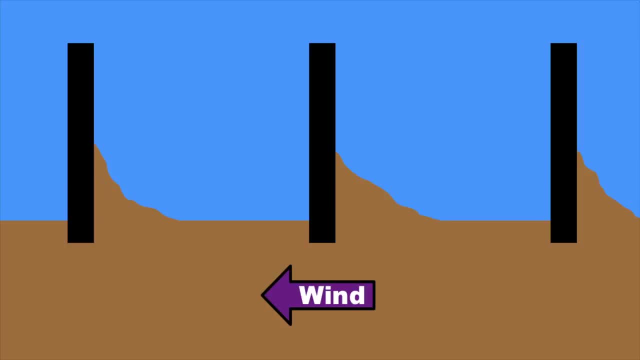 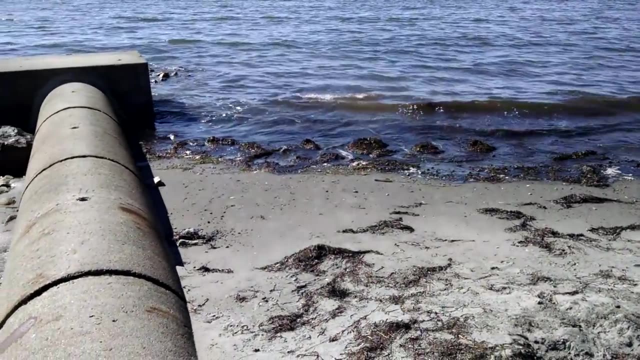 As a result, sand piles up. Sand piles up on one side of the groin, making the boundary between land and water different on both sides of it. This storm sewage outflow pipe acts as a groin. The sand level on one side is higher than on the other. 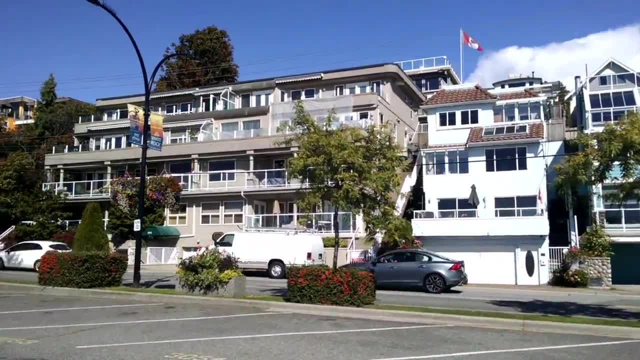 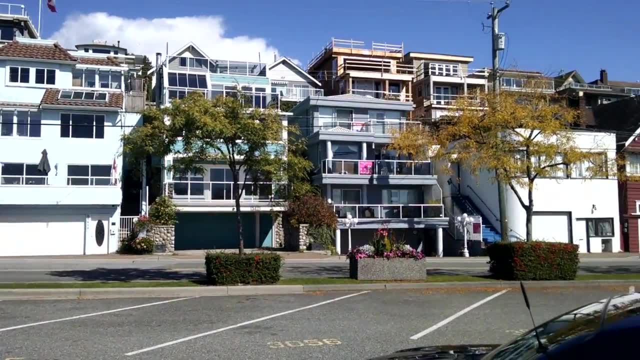 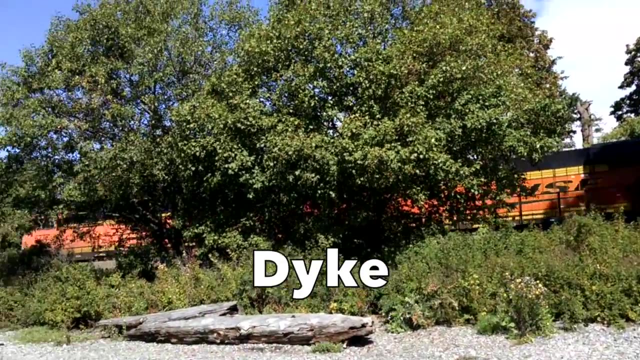 Speaking of storm sewage, our inventiveness has caused us to prepare, by building storm sewage outflow pipes, which basically remove water from the street during a heavy storm and return it to the ocean. On this beach, people have built a dike Which not only holds the railroad tracks but prevents strong waves from making their 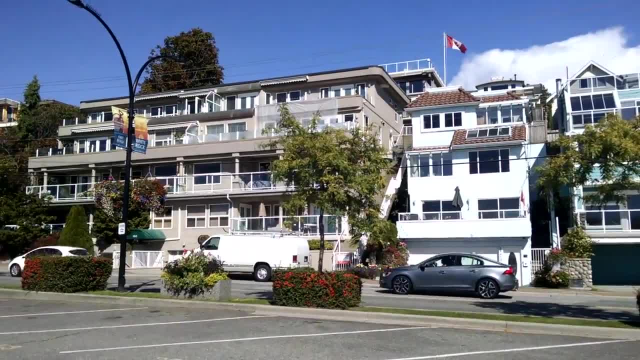 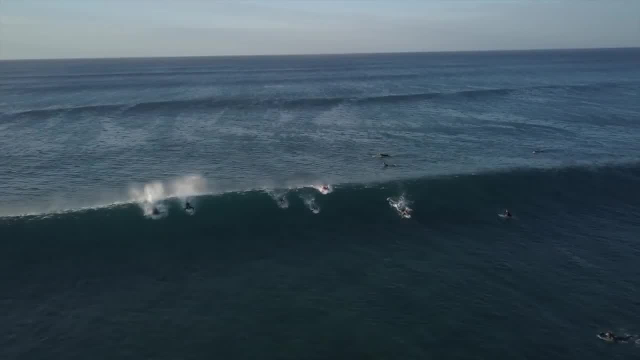 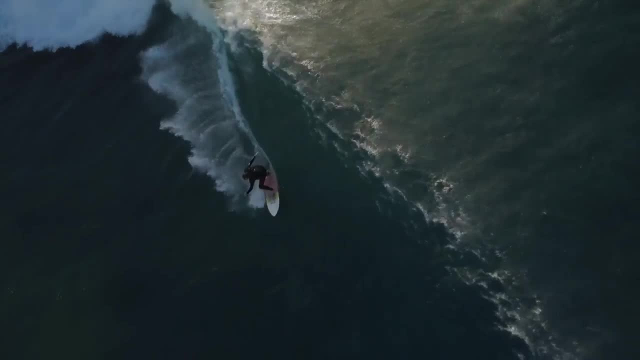 way onto the street preventing floods. The defences here are adequate. the people will live On the note of strong waves. what is a fascinating characteristic about strong waves? They break. Since water travels in columns, the friction of the part near the bottom begins to increase. 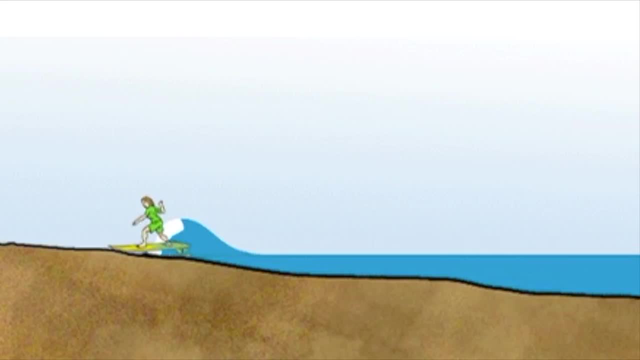 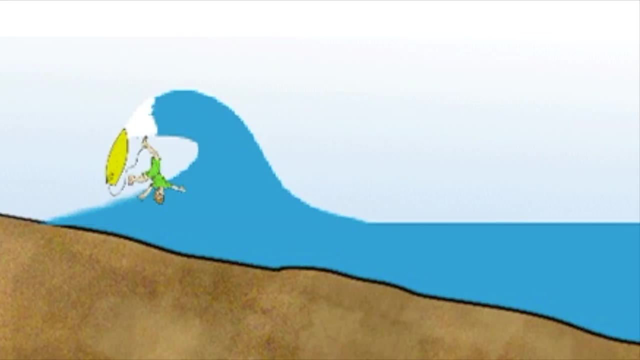 when approaching shallow waters, The bottom part slows down while the top part continues on, Causing the wave to become steeper and steeper until breaking. If the slope of the ground is too flat or too steep, the wave won't break. 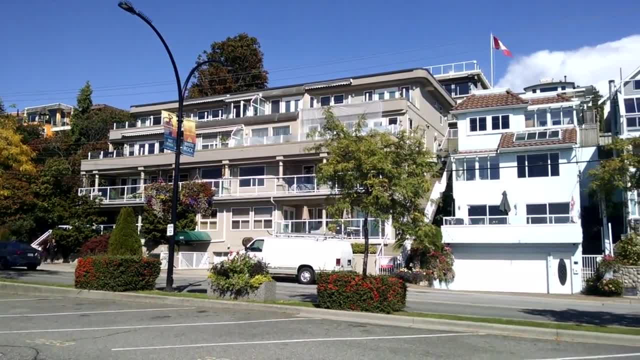 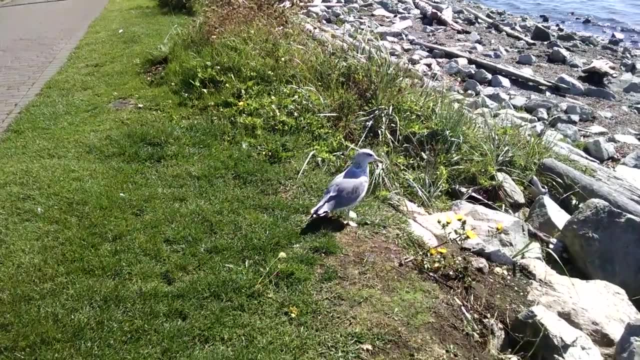 If there were a tsunami here, the only place to go is up the hill. Since this is part of a larger metropolitan area, there shouldn't be a problem with shelter. Another interesting thing here is the wildlife which I got a chance to catch up with. 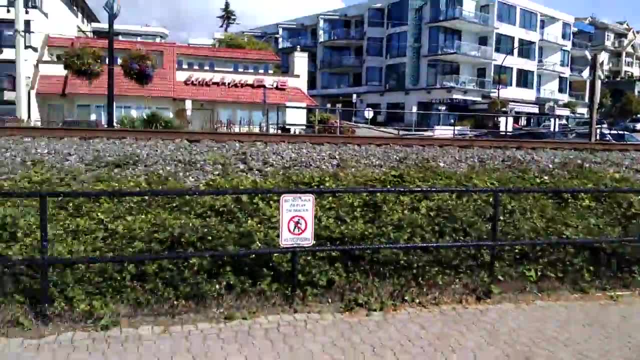 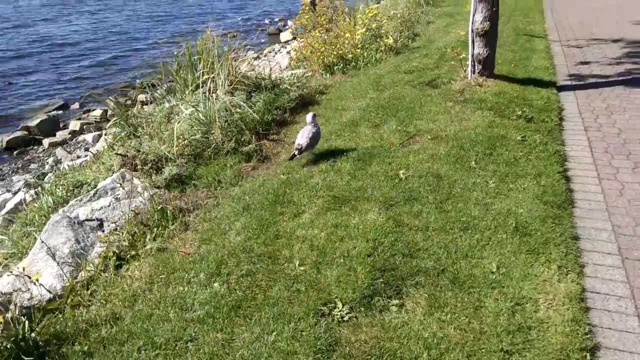 I wanted to get a chance to meet in the nature of the islands, in the middle of dry land. I didn't have time to drop off, so I went ahead and set off to the washed out side. I'm going to take a rest for a while. 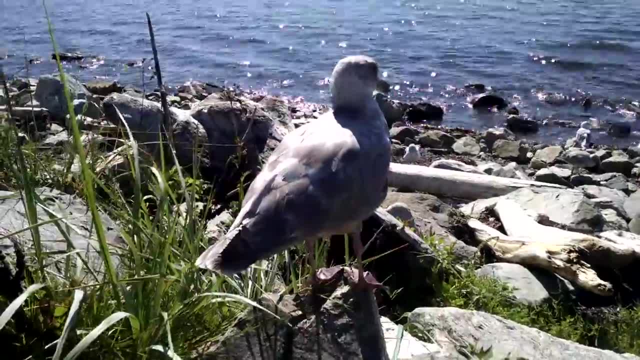 I feel a bit lucky as I'm without a boat, But I don't know how much time this will take, because I have a good understanding of how many people are here, so there's probably a lot of fun and a little bit of a Whether. 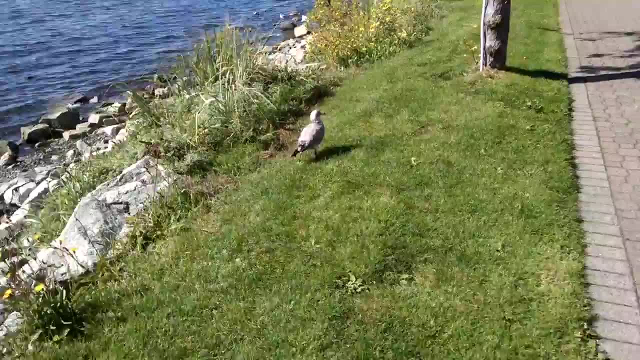 I can catch up with those who aren't. that's a bit of a challenge for me to work with, But that's a silly thing. There are people who might add to that in a minute or two, but the смотрите is very. 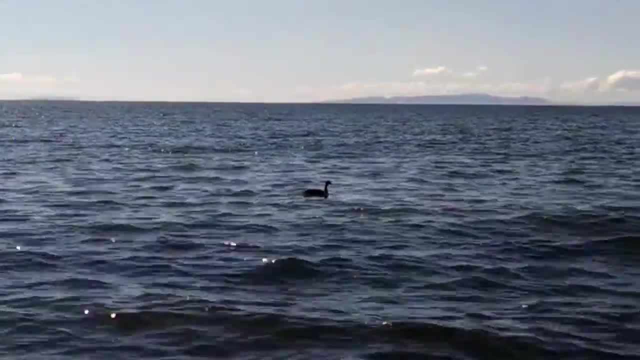 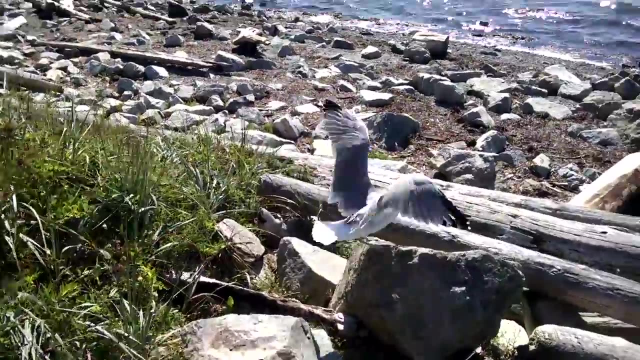 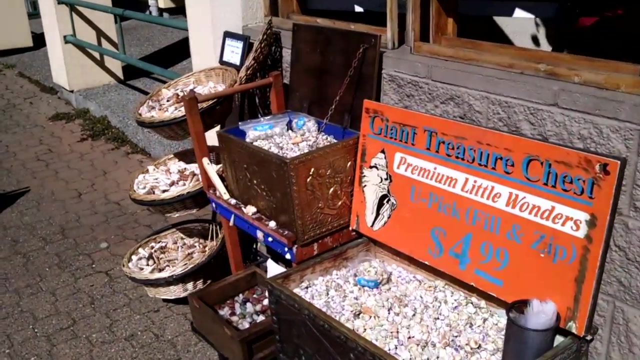 important to me. This is a big project that I'm working on. It's going to take a lot of time. I'll be sure to get my supplies as early as possible. We haven't even considered most of the social aspects of the coast. 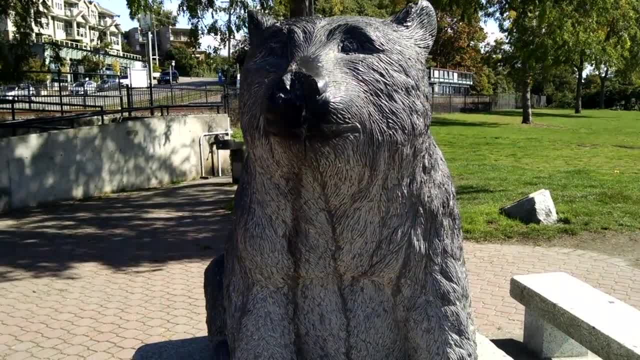 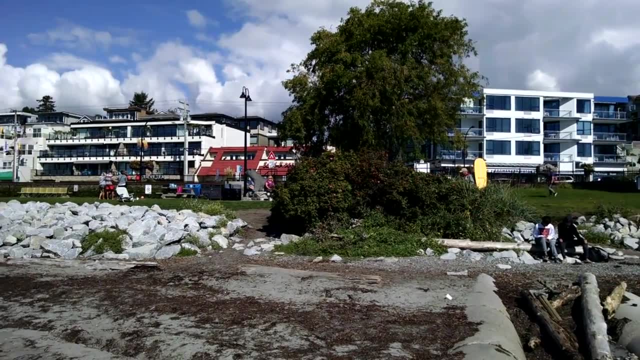 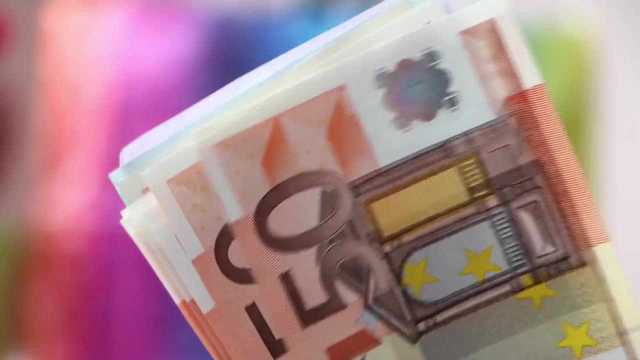 Like this bear with a broken nose. Maybe he got into a fight with a seagull. Ocean front real estate is often quite expensive, Since people like going to the beach for leisurely purposes and people are naturally driven by self-interest. there are many stores and restaurants to accommodate hungry beachgoers. 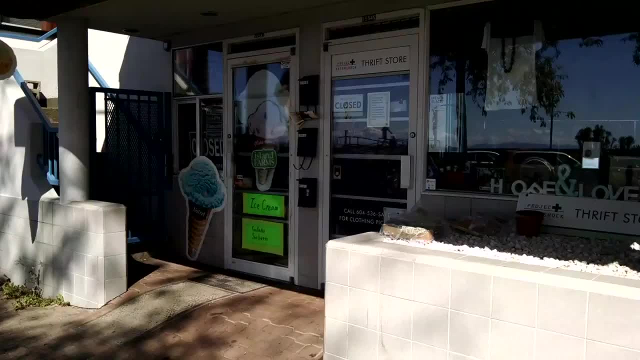 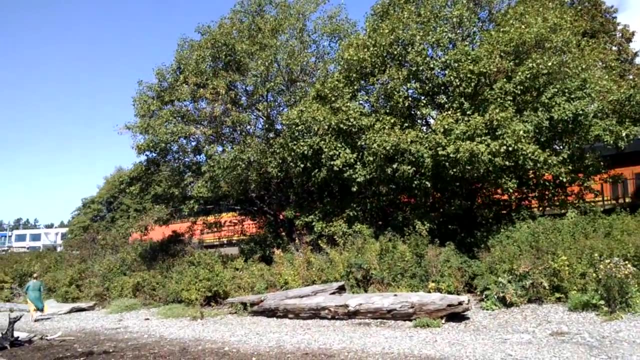 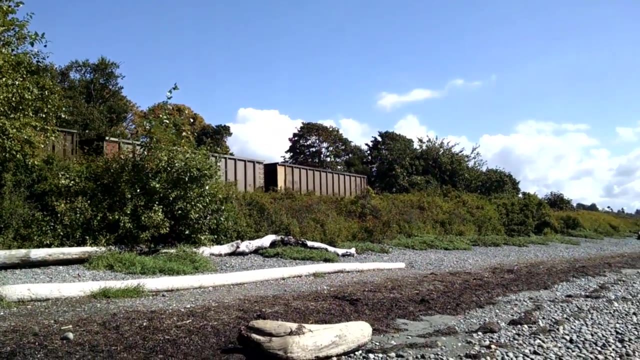 looking for something to eat and those looking for a treat. This area also has a rich history. These railroad tracks, which sit upon the dike, used to serve a railroad station to this community and continue to facilitate trade between British Columbia and the United States, as well as.